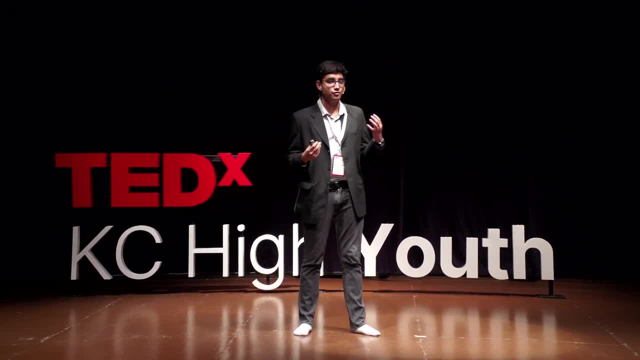 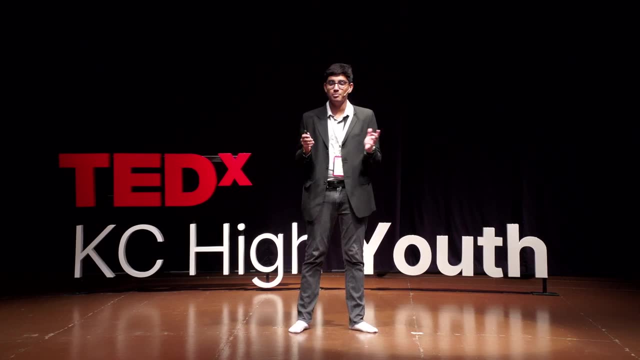 have a certain number of items to be placed in a certain number of containers. but if I have more items than containers, it turns out that at least one container is going to have multiple items. I don't explicitly have to be talking about pigeons in pigeonholes. I could be talking 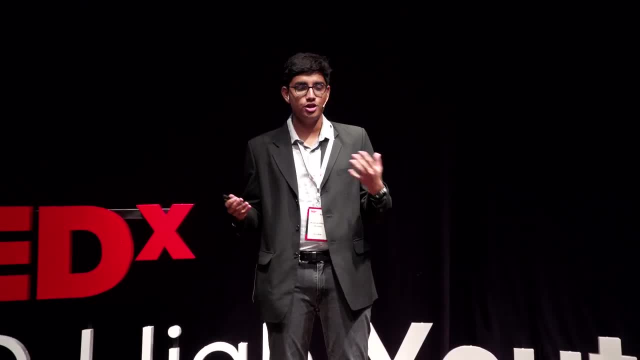 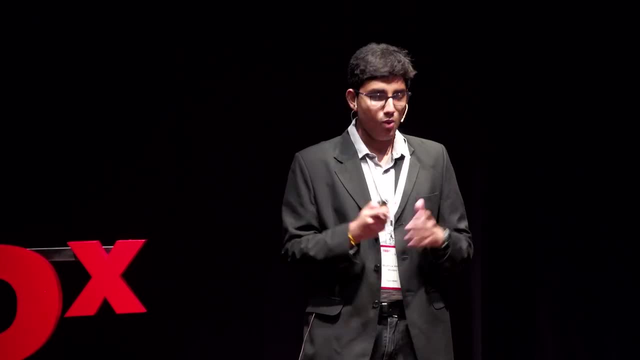 about anything from pencils to pencil pouches, socks to drawers and even the weird example of strands of hair in people's heads, something I'll be getting into in a bit. What's also neat about the pigeonhole principle is that I can extrapolate it to as many items and 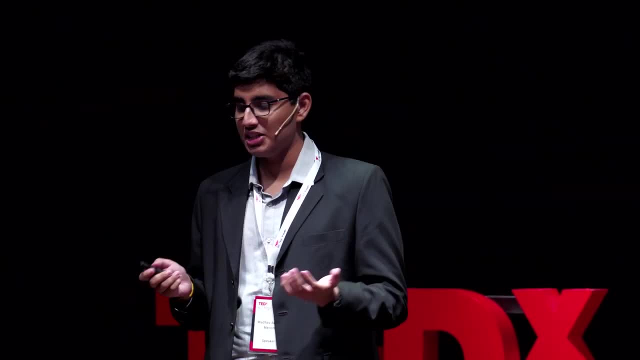 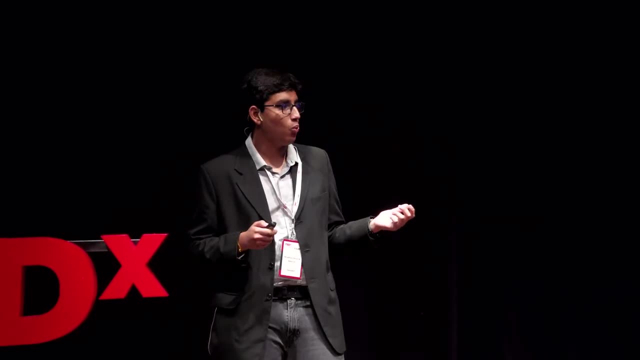 containers as we want. As long as I have more items than containers, I can use the pigeonhole principle. Here we have nine pigeons and four nests, And so if I place one pigeon into one nest at a time and if I group together the surplus, 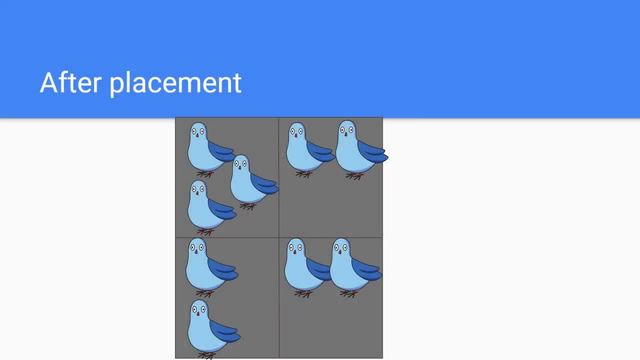 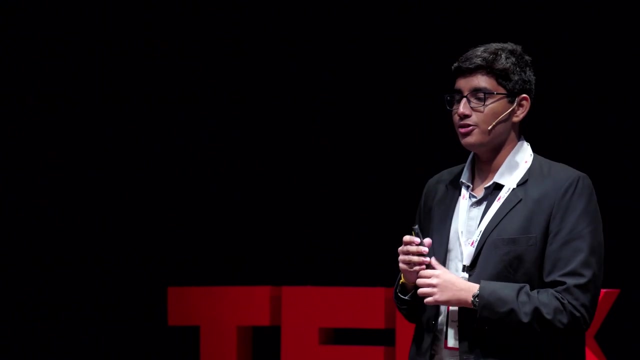 pigeons, I might get something that looks like this: Since we had more items than containers, the pigeonhole principle said that at least one container must have multiple pigeons, And over here, all of our containers have more than one pigeon. I want to digress a bit and introduce a mathematical concept, But trust me, it's very simple and 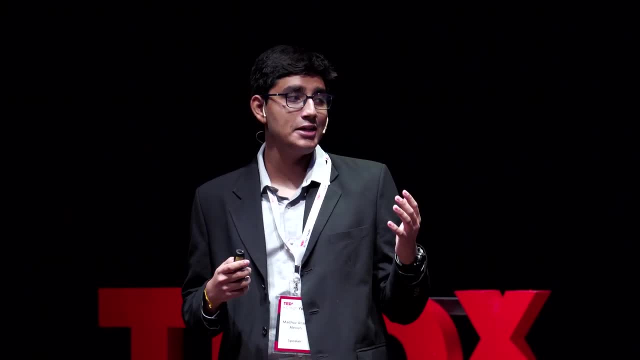 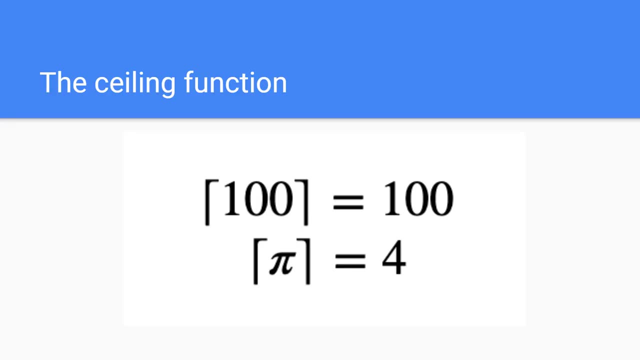 it's called the ceiling function. Without it, it would be hard to get into the nitty-gritties of the pigeonhole principle. The ceiling function is very simple and is noted by these weird-looking brackets that point towards the ceiling. Effectively, all it does is take in a number and give you an. 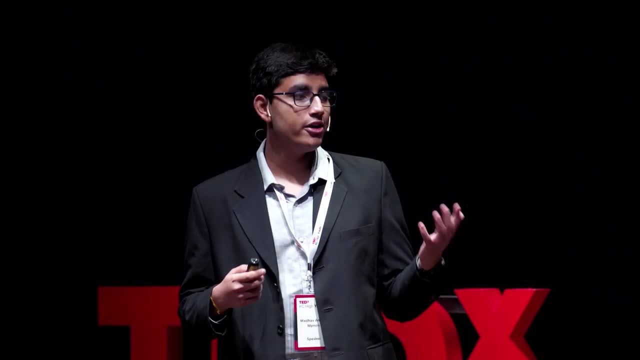 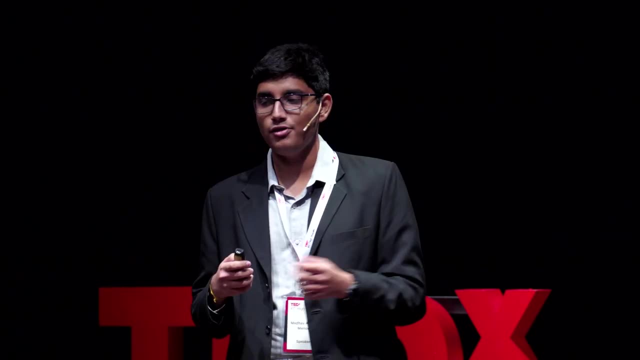 output. The output is another number that is the nearest whole number greater than or equal to the number you gave it. A hundred is already a whole number and therefore the ceiling function of a hundred is just a hundred. Pi is approximately 3.14, and therefore the 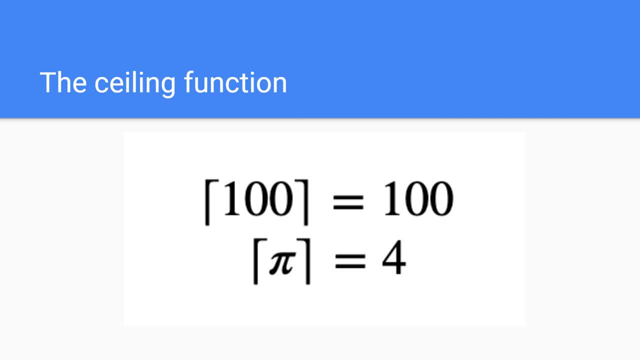 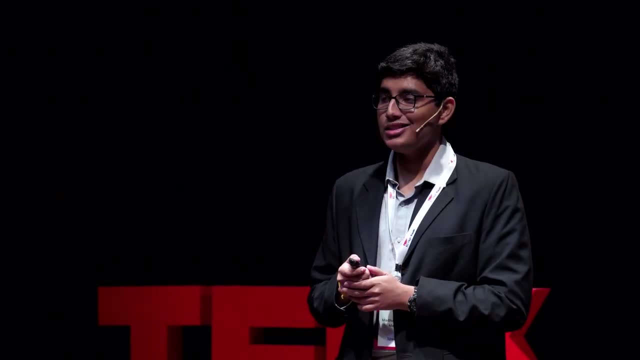 nearest whole number greater than or equal to 3.14 is the nearest whole number greater than or equal to 3.14.. So the ceiling function of pi is 4.. Now why did I bother introducing this to you? The reason is that we can actually formalize. 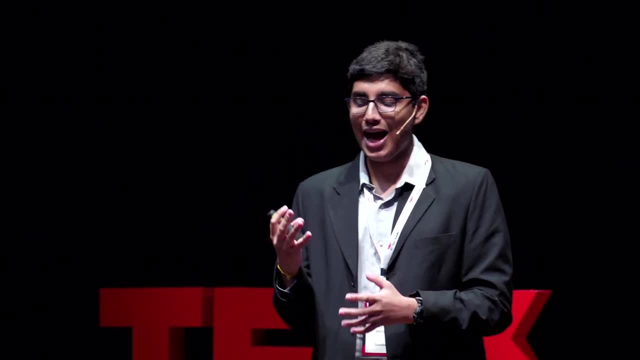 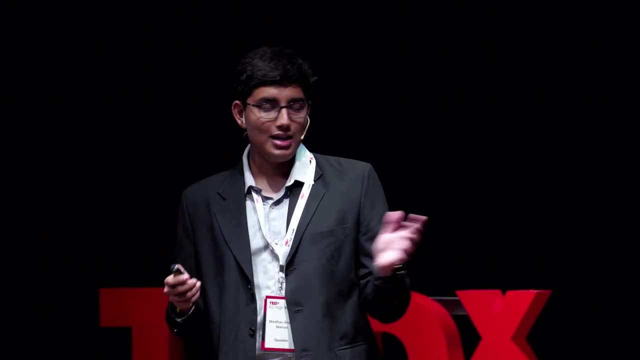 the pigeonhole principle a bit. If I know exactly how many items in containers I have, I will get an idea of approximately how many items there will be in a given container. Let's rephrase the pigeonhole principle a bit. Looks pretty complicated, but effectively. 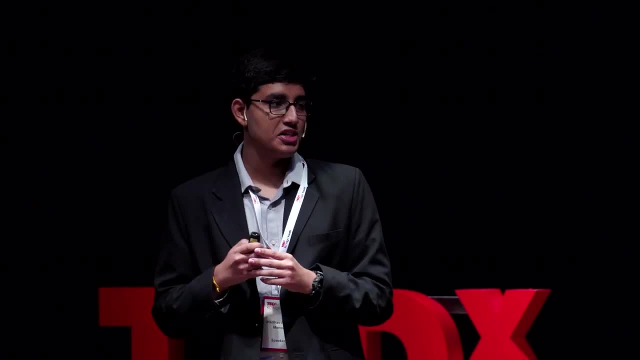 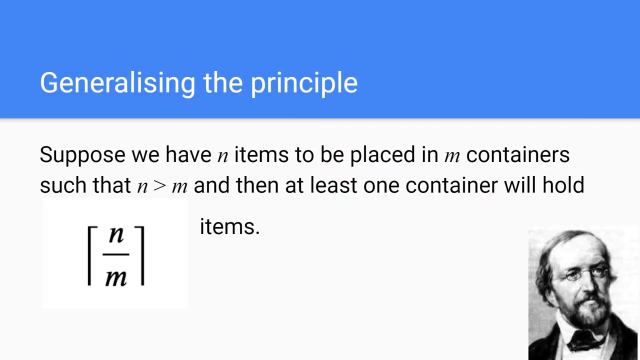 if I have a certain number of items to be placed in a certain number of containers and if I have more items in each container, I will know that the number of items to be in containers- at least one container- is going to hold the ceiling function of the number. 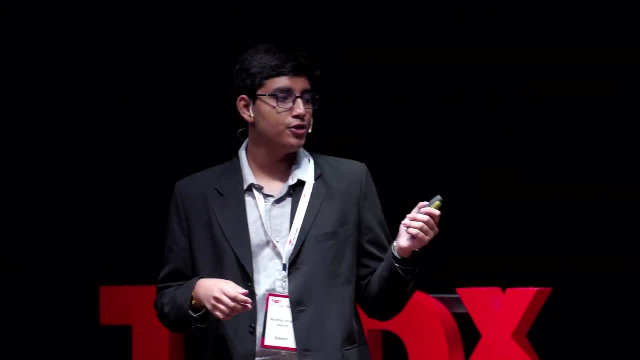 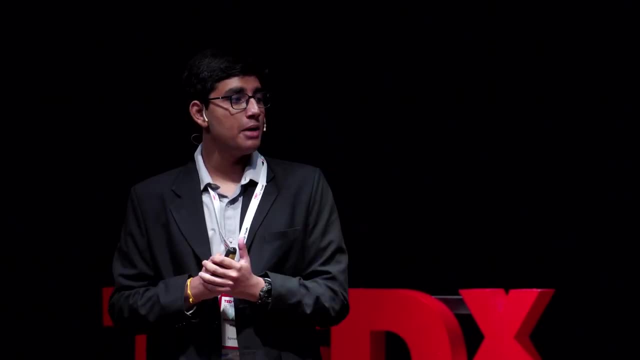 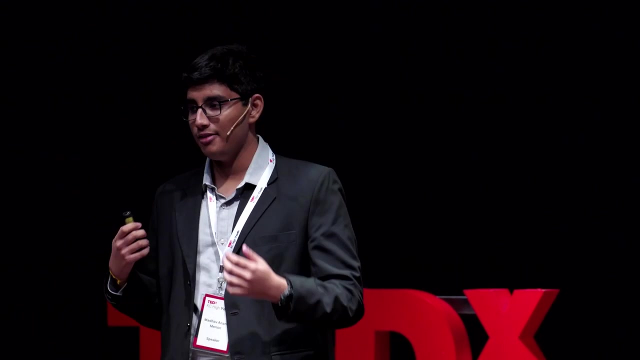 of items divided by the number of containers Sounds confusing. Don't worry, we'll illustrate it with an example. This formalization came about by the French mathematician Jean Larochon in a book he wrote in 1622.. However, it's now more widely attributed to the famous German mathematician Peter Gustav. 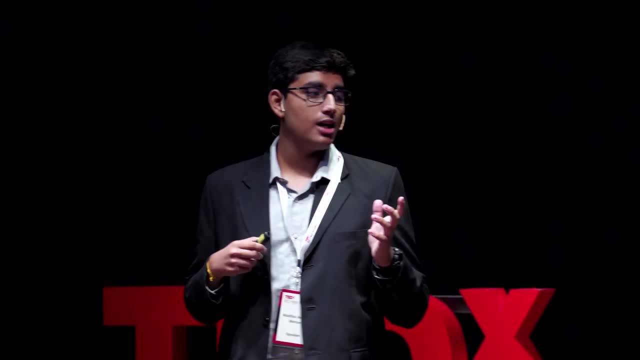 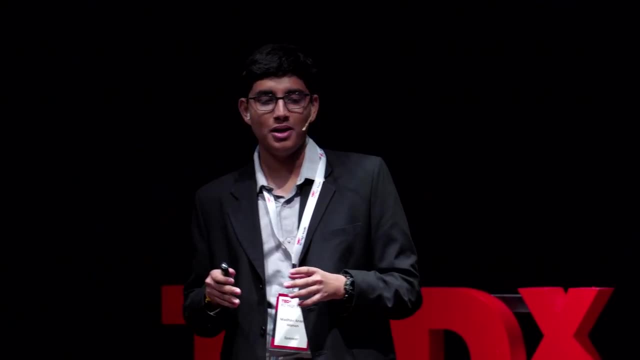 Legend de Leclerc: The beauty of mathematics comes from how you derive principles and theorems from the basic axioms that govern mathematics. But this talk is not about deriving the pigeonhole principle, so I want you to take this for granted. 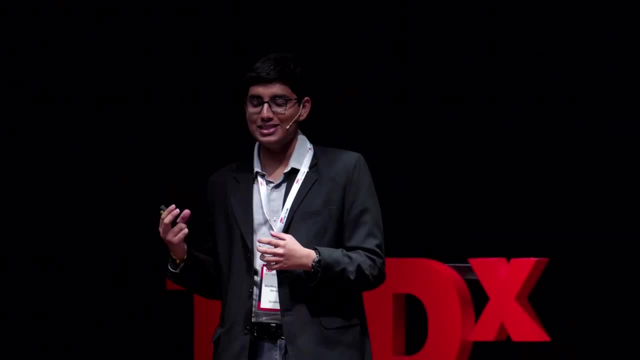 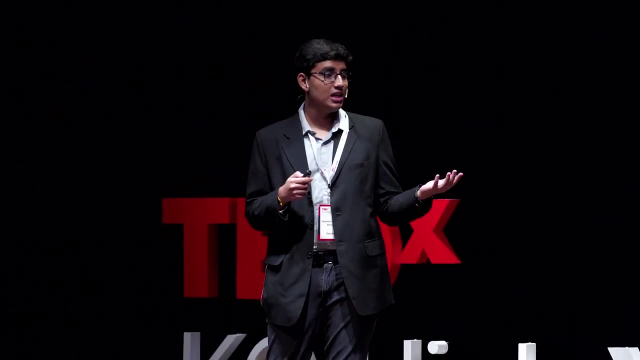 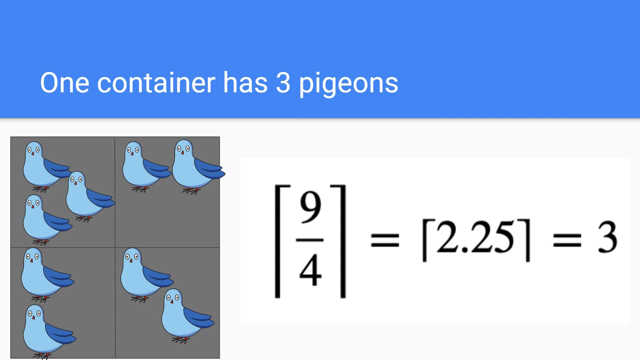 Instead, we're going to look at how such a simple idea of placing items into containers can be used to understand some pretty important ideas around us. Let's go ahead and illustrate the pigeonhole principle with our previous example. Here we had nine pigeons, or nine items and four containers. 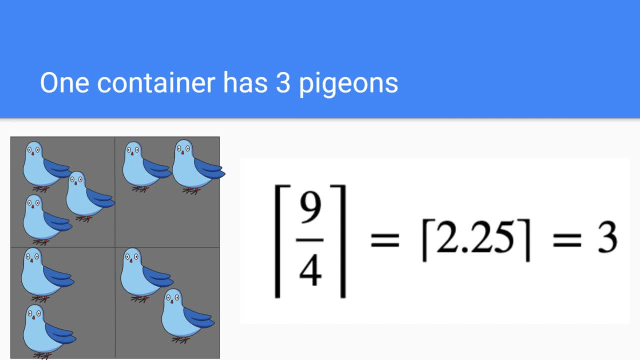 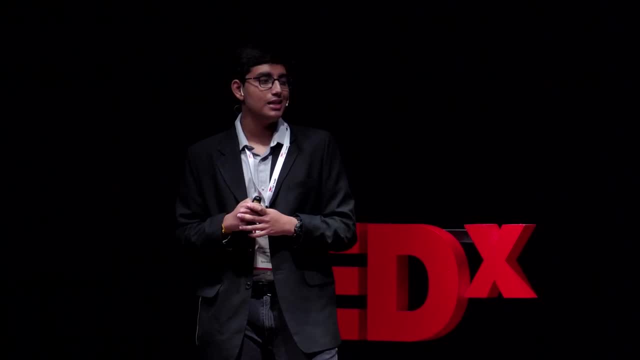 And therefore one container is going to hold at least the ceiling function of the number 9 divided by 4.. Nine divided by 4 is 2.25. And therefore the pigeonhole principle states that at least one container is going to hold. 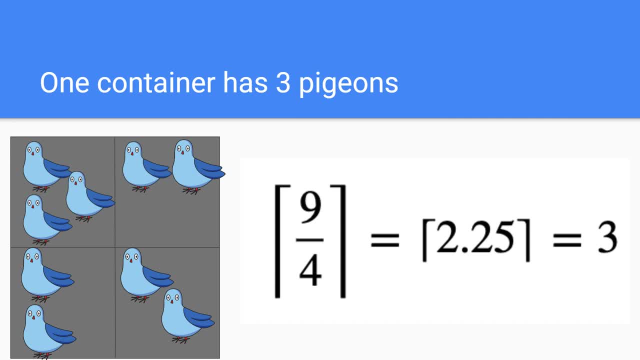 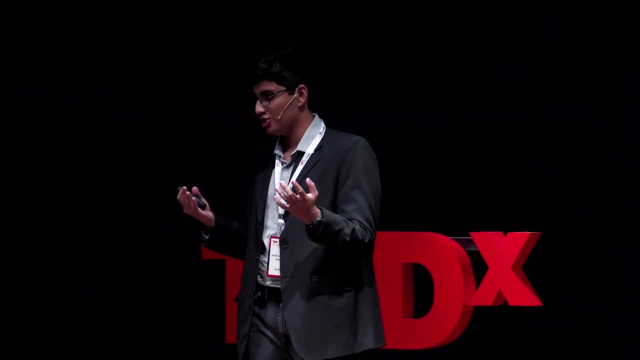 the ceiling function of 2.25,, which is 3.. Over here you can see that one container holds exactly three pigeons. Holding exactly three pigeons and holding at least three pigeons are kind of different concepts. So how do we reconcile the two? 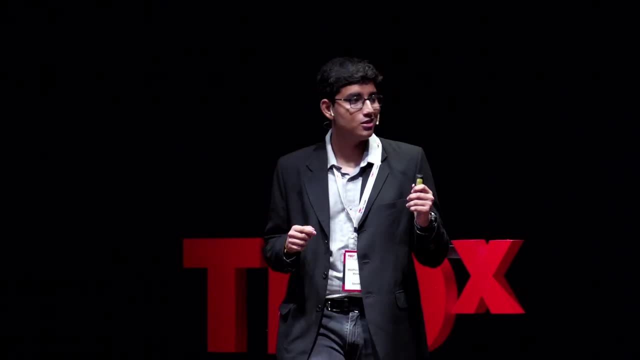 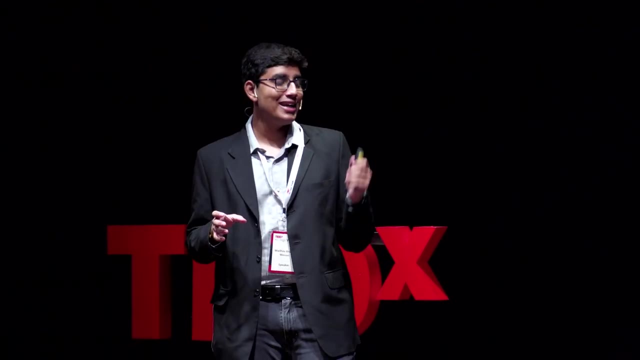 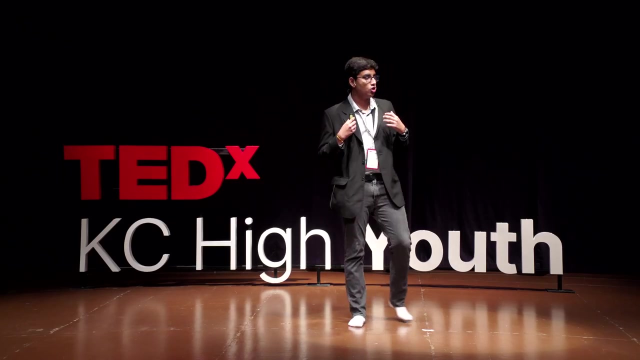 The thing about the pigeonhole principle is that it does not actually take into account different configurations. They're all completely valid as well. Regardless of which configuration you choose. at least one container or at least one nest has at least three pigeons. And this is the idea of the pigeonhole principle: sorting items into containers. 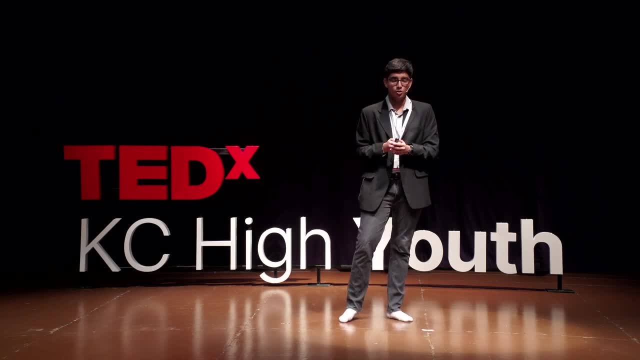 But now that we have a rudimentary understanding of what the pigeonhole principle is, why do we need such an intuitive and common sense idea? The interesting thing about the pigeonhole principle is that it can be used to answer some pretty trivial questions that no one's going to bother us with. 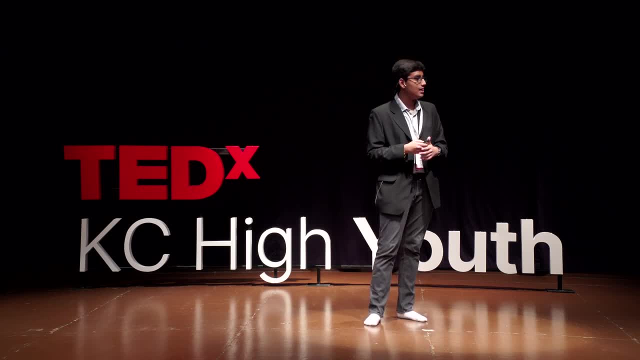 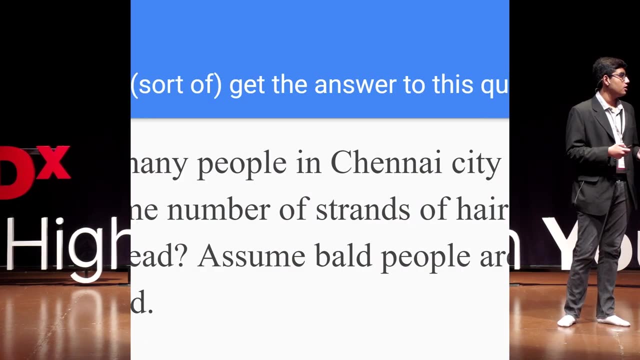 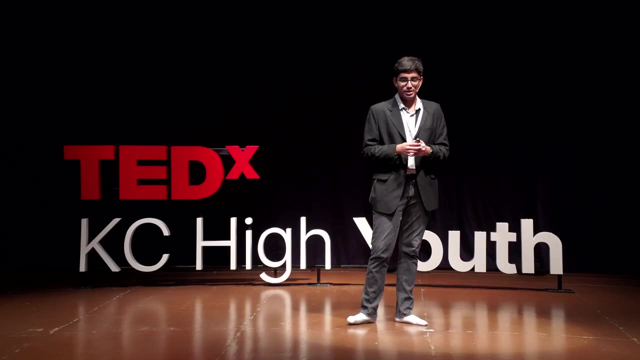 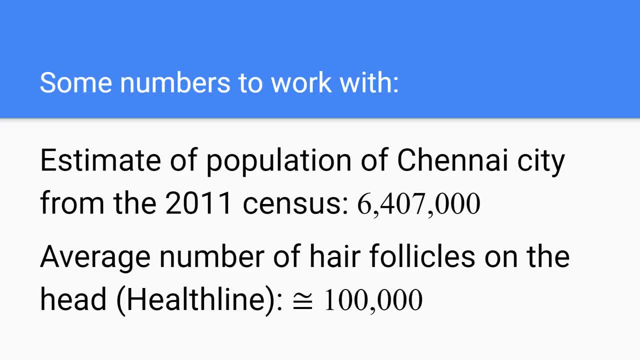 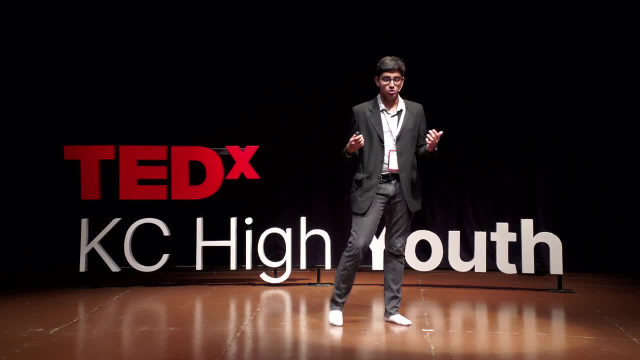 hair follicles on a person's head is approximately 100,000.. Now, this idea of strands of hair and people's head was how Larachan introduced the idea of the pigeonhole principle as well, although he did not use Chennai city. So how do we use the seemingly innocuous idea of sorting items into containers and apply? 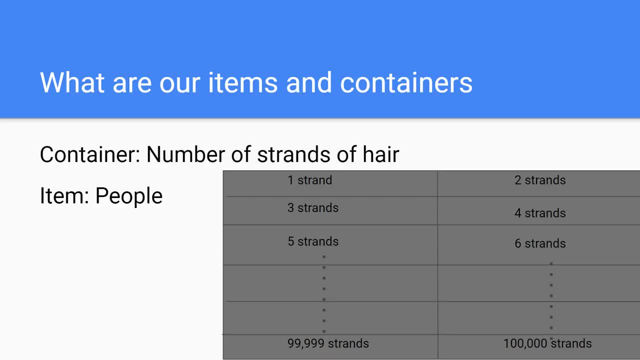 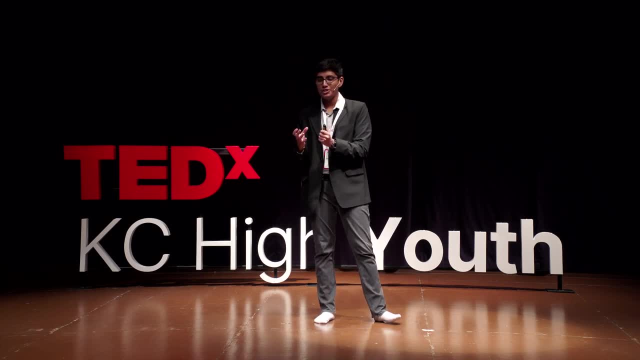 them to strands of hair and people's head. We can, if we think outside of the box a bit, Imagine that our containers are like a box. The containers are like the number of strands of hair, our hair follicles. For example, one container could hold all the people with just one strand of hair on the 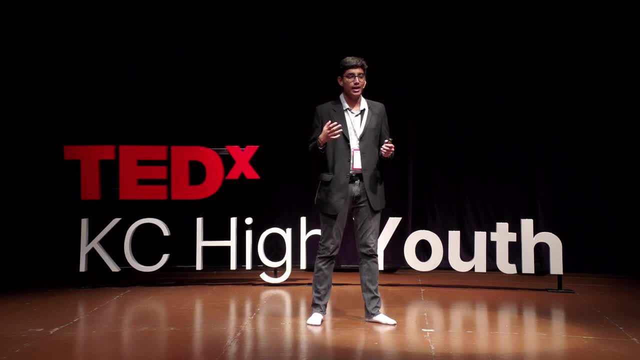 head, The second container, all the people with two strands of hair, so on and so forth. And if we think about our items as the number of people and if we place them according to the number of strands of hair on our head, we can effectively use the pigeonhole principle. 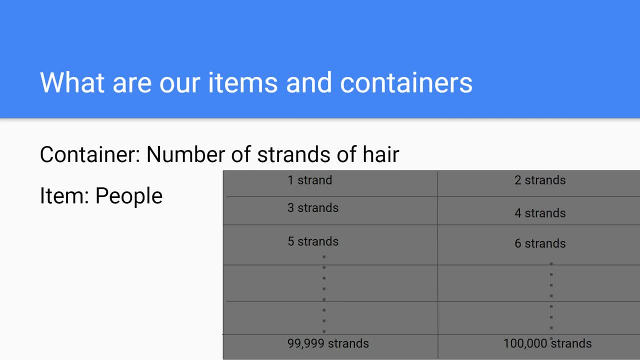 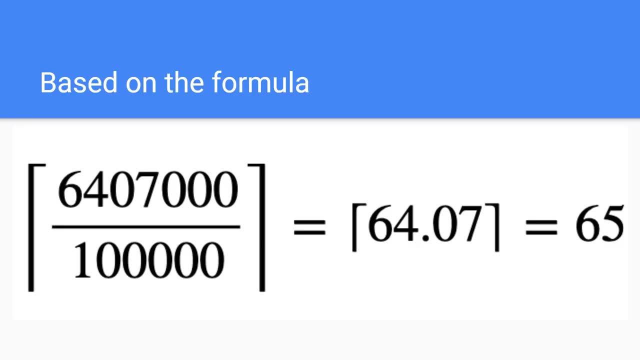 Here we have 100,000 containers, but we have 6,407,000 items. We can effectively use the pigeonhole principle. apply the pigeonhole principle, we would get that there are approximately 65 people in China, or there are at least 65 people in China with the same number of strands of. 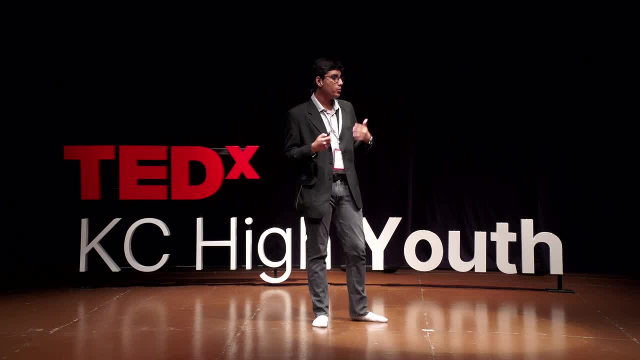 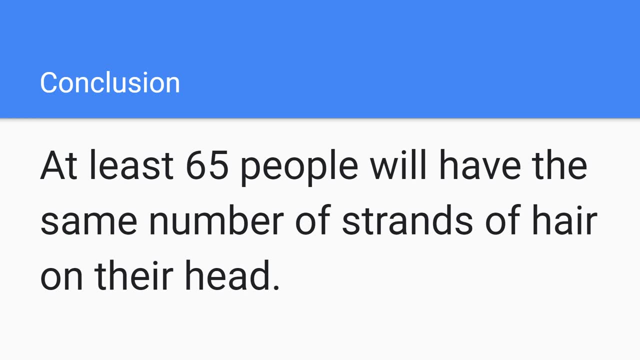 hair on their head. But this is pretty useless, right? Why do we care about the number of strands of hair on people's head? And this number doesn't really tell us anything about the actual number of strands of hair these 65 people have. So let's look at something. 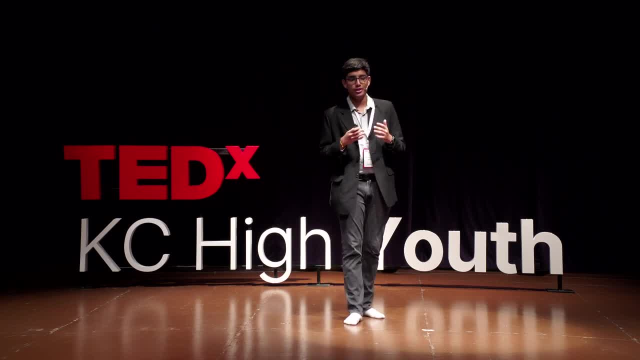 a bit more relevant in our day and age. Let's look at something in computer science: the idea of data compression. We've all dealt with data compression on a day-to-day basis. We have a really large file that we want to send to someone, but we just can't because 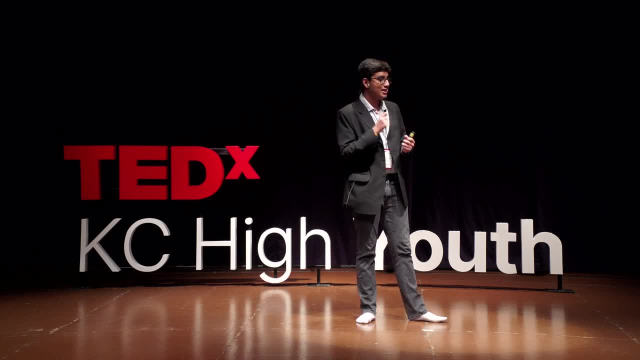 it's too big, So we go ahead and compress that file and make it smaller so that we can send it to our friends and family. It turns out that there are two types of compression. We have lossy compression and lossless compression. Lossy compression is where certain pieces 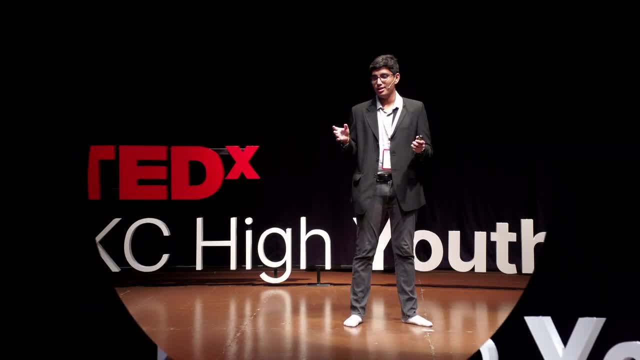 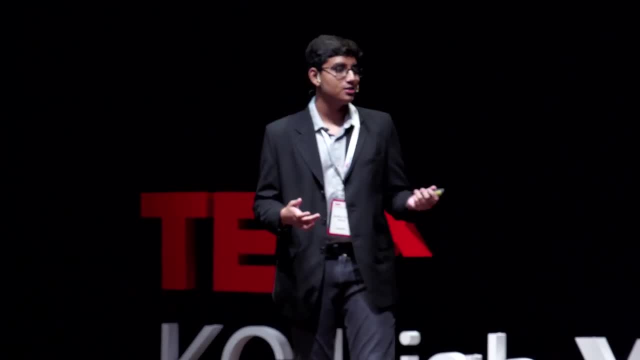 of redundant information are completely taken away from the file. If we have a video, we can't see the audio. Perhaps certain audio frequencies we can't hear are removed. If we have an image, certain colors our eyes can't perceive are removed as well, Effectively. 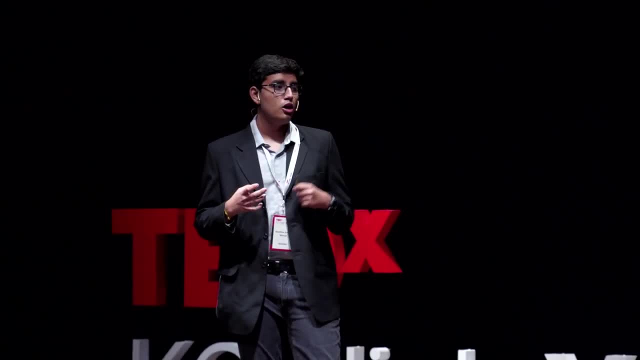 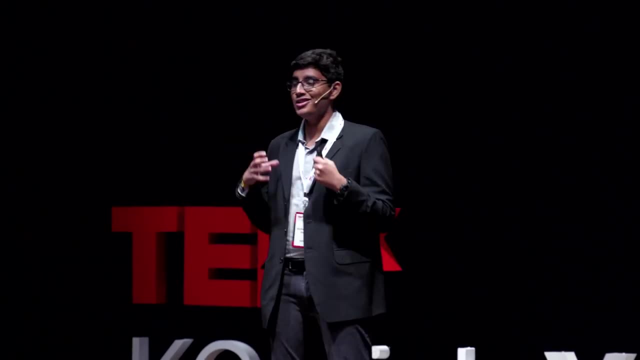 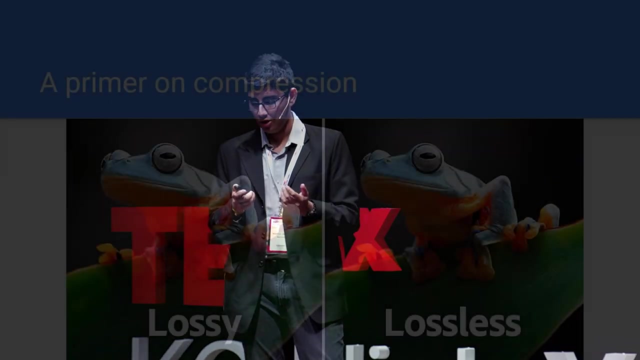 lossy compression involves removing information. Lossless compression, on the other hand, does not remove any information at all. Instead, lossless compression identifies underlying patterns within the data that we have something called statistical redundancies, and it exploits these to make our files smaller. In fact, you can see that the frog that underwent lossless 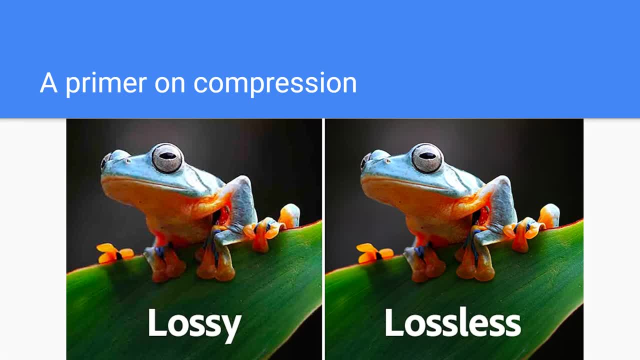 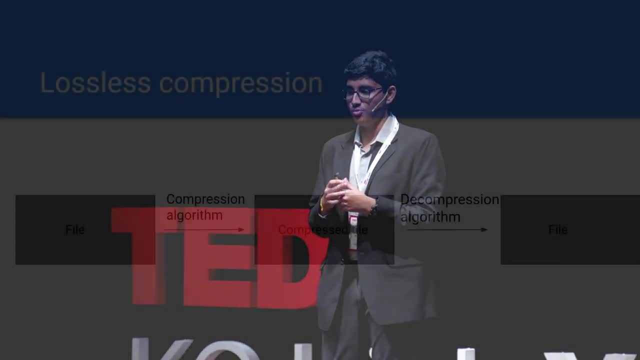 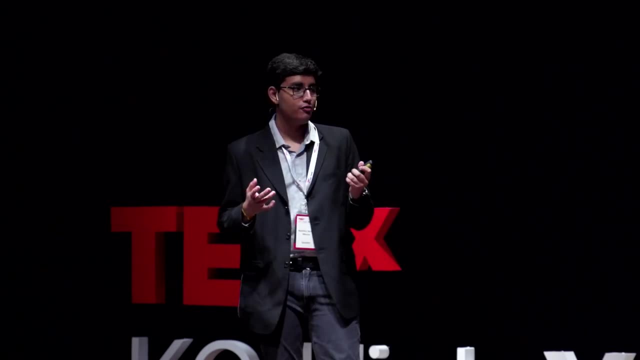 compression is not as blurry as the frog that underwent lossy compression. That's because no information was really removed from it at all, And so, if no information was removed, I should ideally be able to get back my original file, since it's still faithful to what the original file was. If I apply my compression algorithm to a file, I should be able to get a compressed file, But since no information was removed, if I decompress that file, I should be able to get my original file back again. This seems extremely ideal, right? 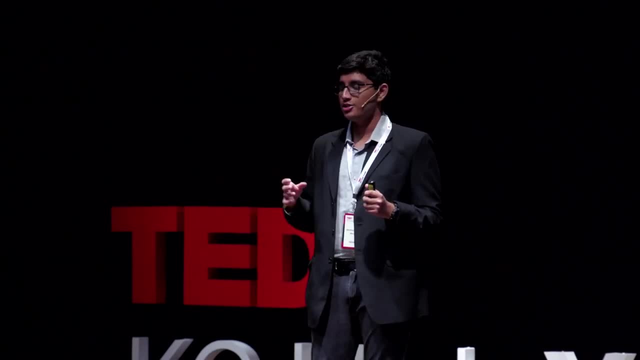 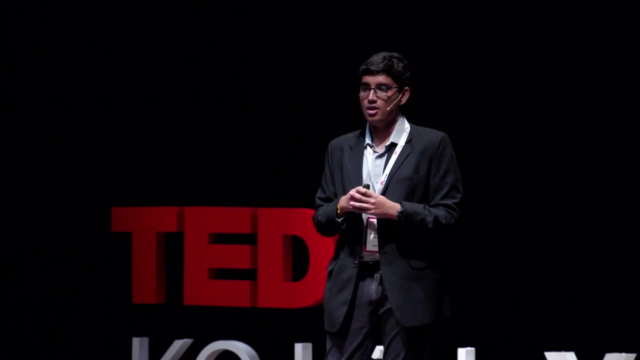 Imagine if I was sending some pretty important financial information to someone all the way at the other end of the world. I wouldn't want any data lost and therefore I would want to use lossless compression. But unfortunately our world is not ideal and there are certain constraints. 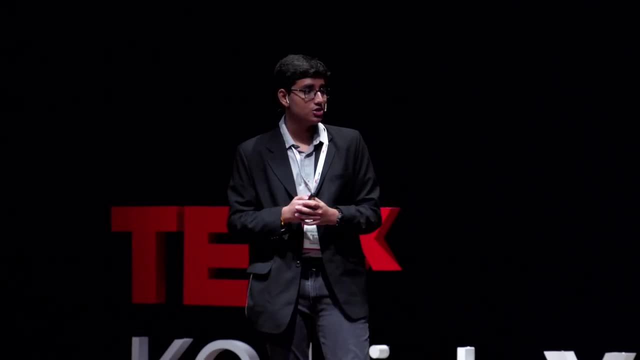 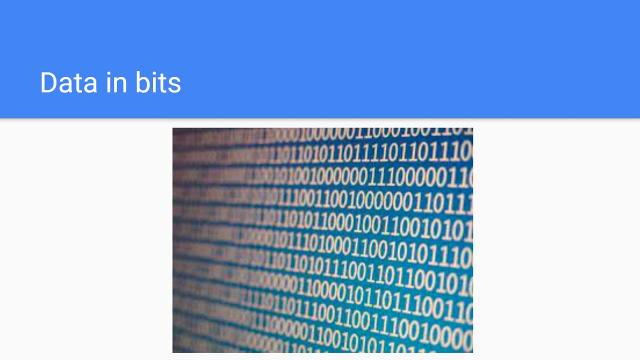 And the pigeonhole principle can be used to identify the certain constraints that we have with lossless compression. But before that, another interlude: All the data we have is not the same. All the data we have in the world is stored as tiny ones and zeros, bits. 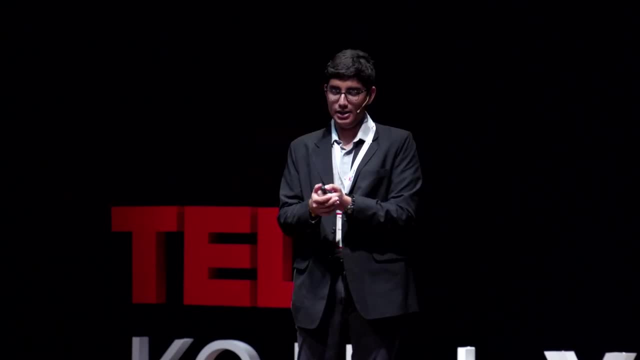 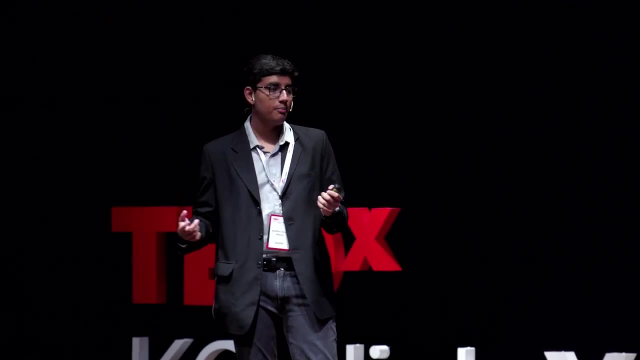 Together. they can collectively be known as binary, a term you might be familiar with. The size of a file is simply dependent on the number of ones and zeros we have, or the number of bits. For example, a two-bit file might look like this: 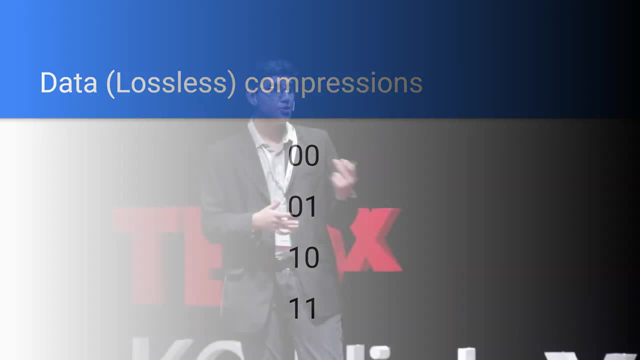 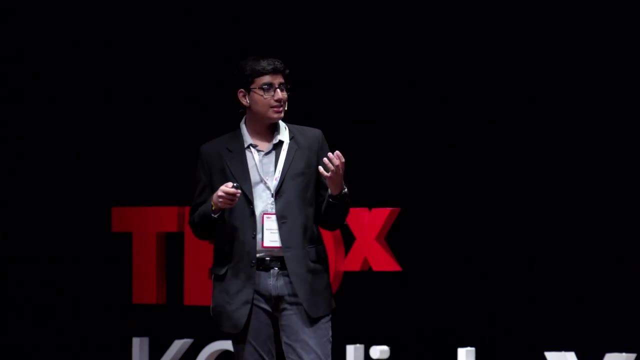 The reason it's a two-bit file is because we have two bits, two combinations of ones or zeros, And these are all the possible combinations we could have for a two-bit file. But let's say I want to compress this two-bit file into a one-bit file. 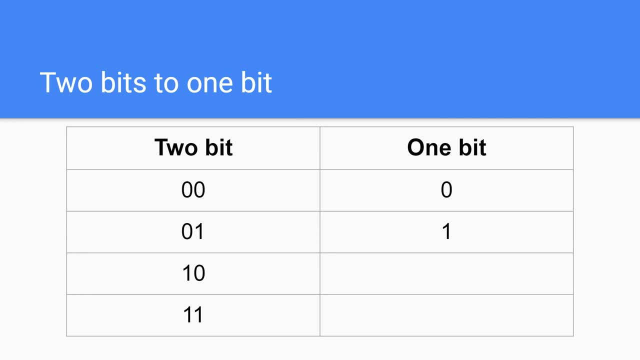 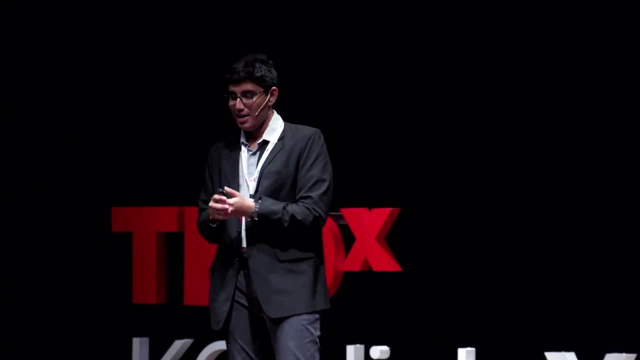 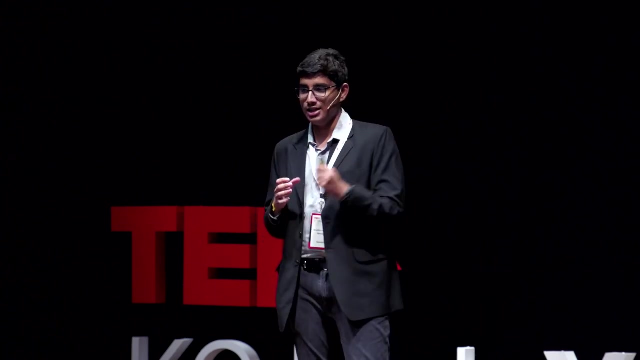 There are only two possible one-bit files. I either have a zero and a one, And therefore I'm effectively mapping four possible files to two files. How do we apply the pigeonhole principle If we once again think outside of the box and think of our one-bit files as the number? 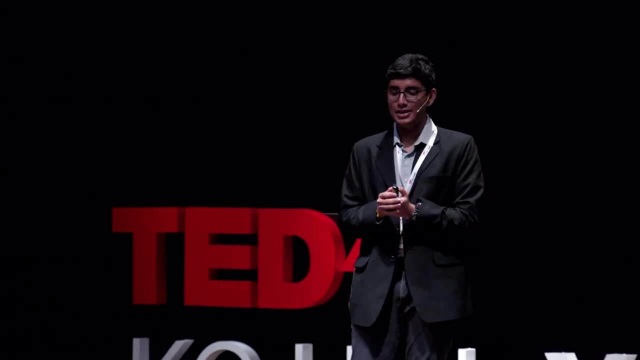 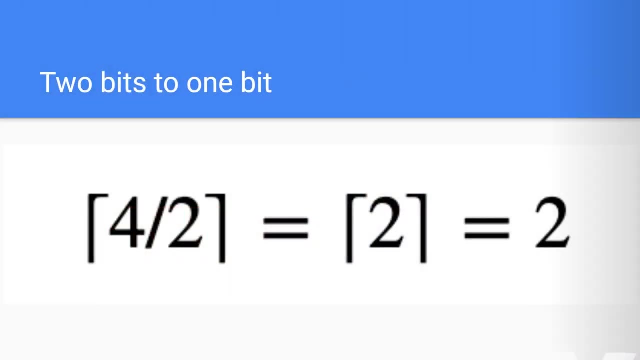 of containers, while our two-bit files as the number of items. we're effectively trying to sort four items, All right. All right, So I have two specific containers, And so if I apply the pigeonhole principle again, I get that there must be at least two. 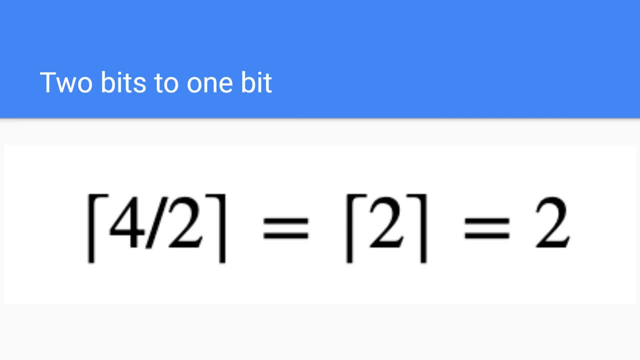 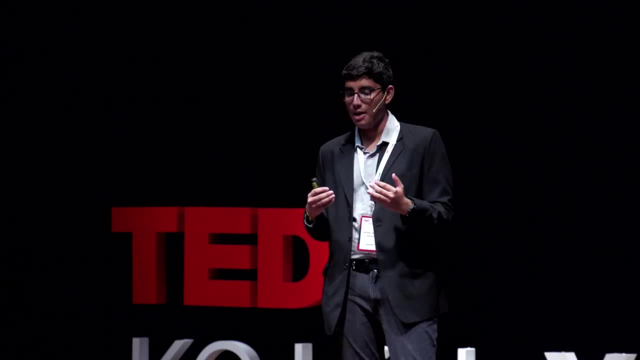 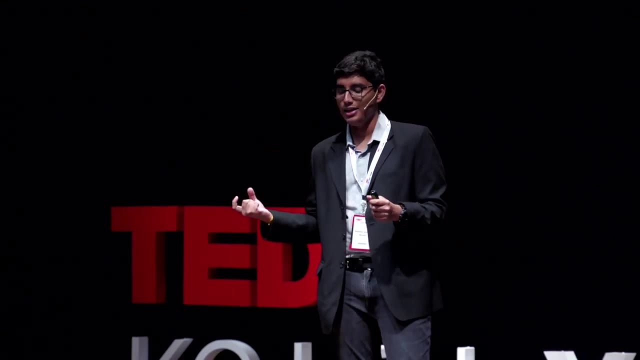 files, two of these two-bit files that correspond to a single one-bit file. Now, this violates losses compression because ideally I should have a one-to-one mapping. I should have one specific two-bit file mapping to one specific one-bit file so that I can. 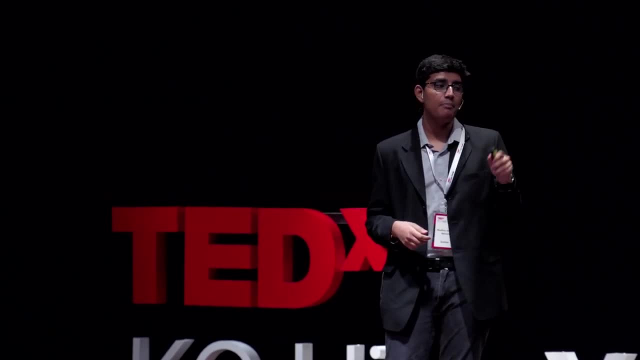 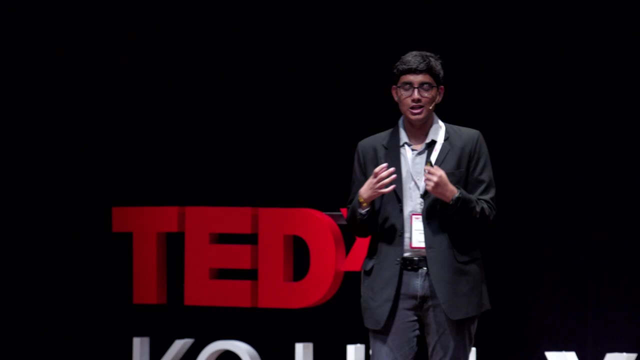 get my original file, But if I have two of these files mapping to just one file, I should have one specific one file. How can I get my original file? Therefore, the pigeonhole principle tells us that there are certain collisions when it comes to lossless compression. 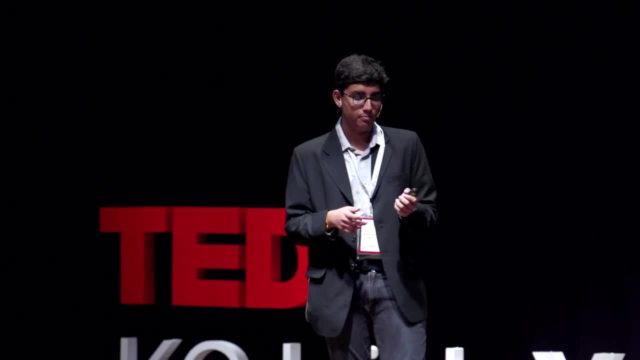 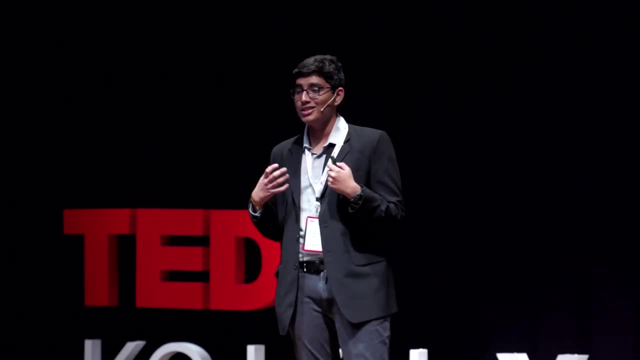 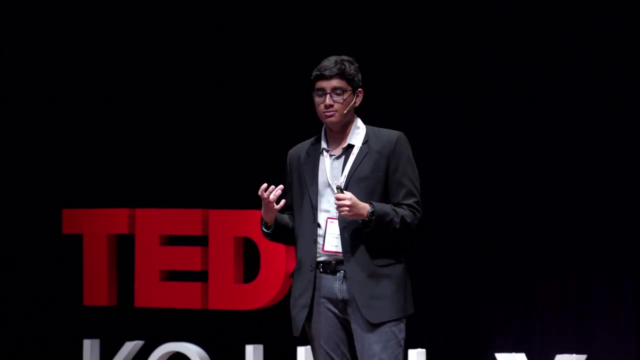 Effectively lossless compression does not work for certain types of inputs And with the pigeonhole principle, we've been able to identify certain constraints in the tools that we, as a human race, have created. The pigeonhole principle is very simple. I'm simply trying to sort items into containers. 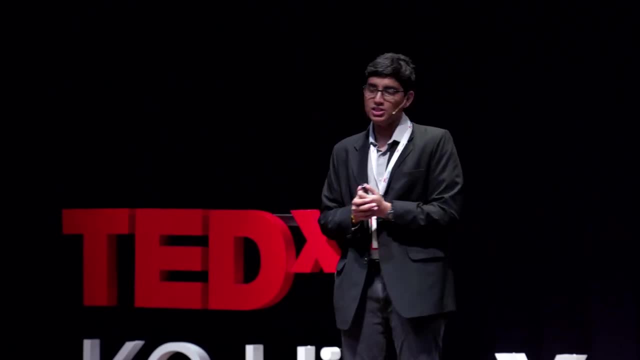 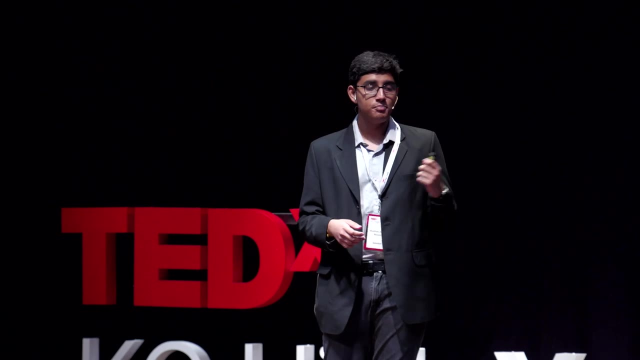 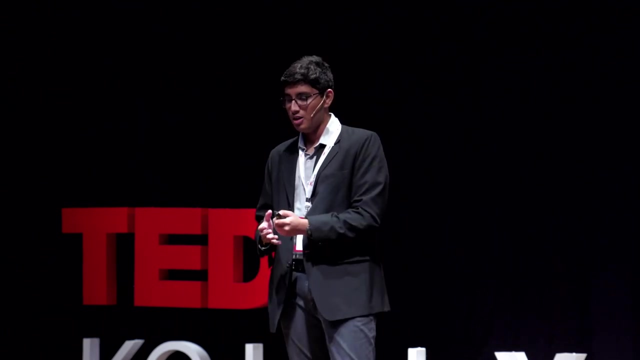 It's so intuitive And it just makes so much sense that perhaps it doesn't need to be formalized as a mathematical principle. Yet it has its applications elsewhere, from it being used extensively in mathematical proofs to other fields of computer science like data encryption and hashing. 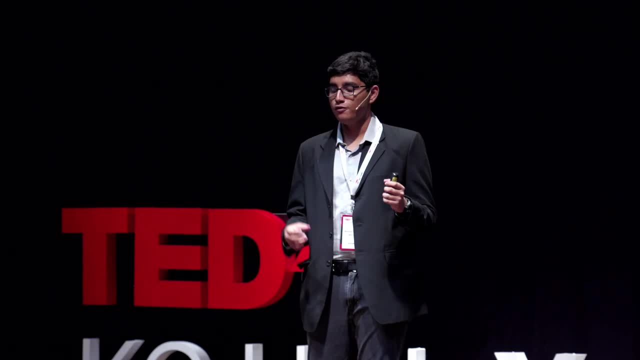 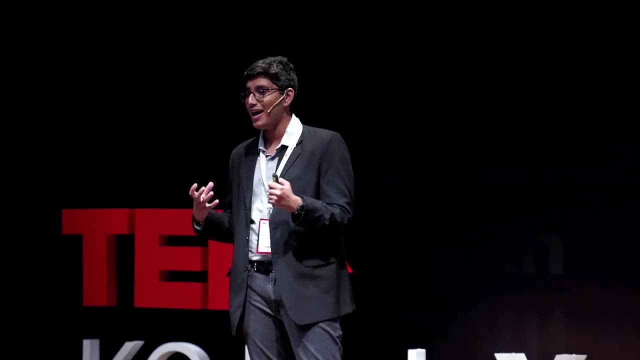 But how exactly do I go from such a small idea of sorting items into containers to having such a big impact on the way we deal with technology, the way we interact with it? How do I bridge this divide? How do I bridge this gap? 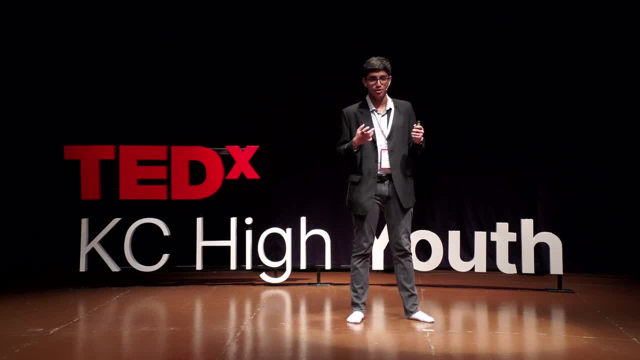 Sometimes it's all about identifying the pigeons in the pigeonholes. Thank you very much.